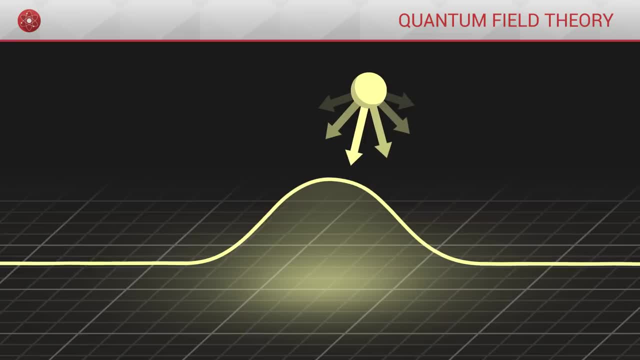 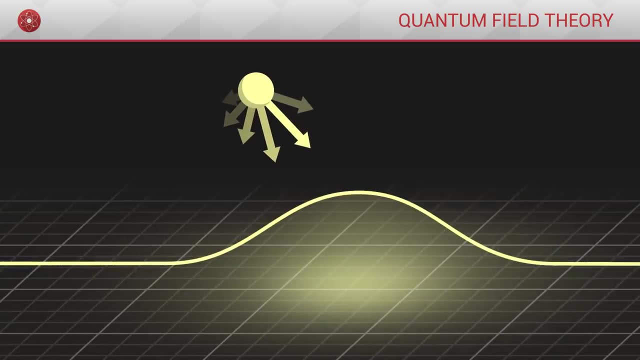 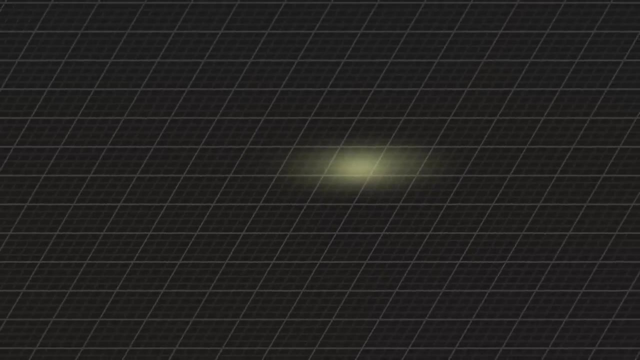 Quantum mechanics allows us to describe the evolution of a particle over time. However, this description, as effective as it is, fails to take into account two considerations. Firstly, quantum mechanics cannot describe situations where the number of particles varies over time. However, quantum mechanics cannot describe situations where the number of particles varies over time. However, 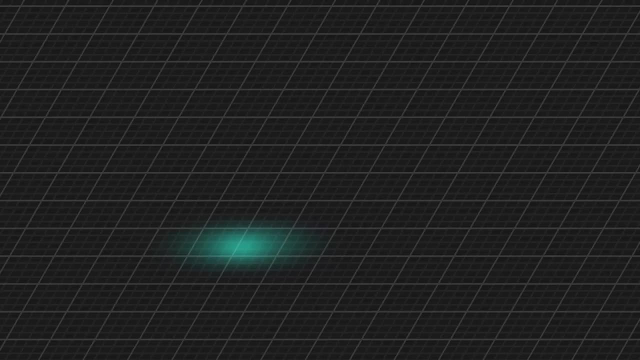 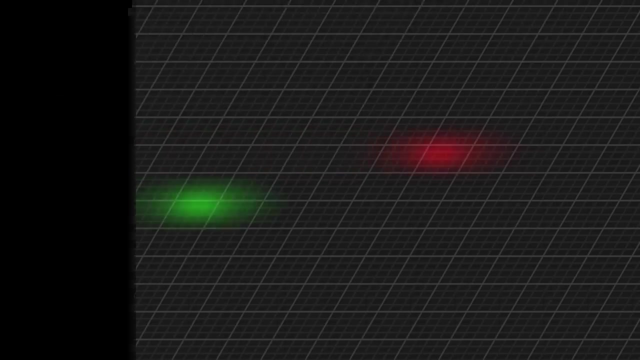 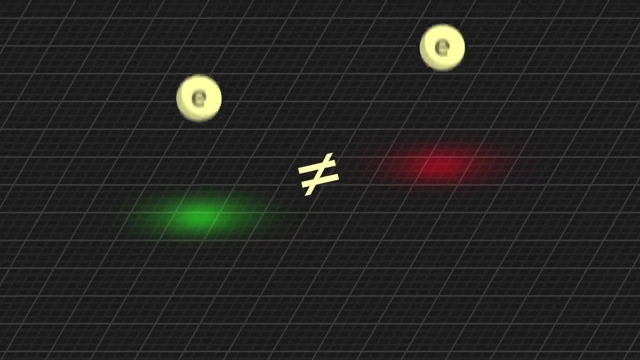 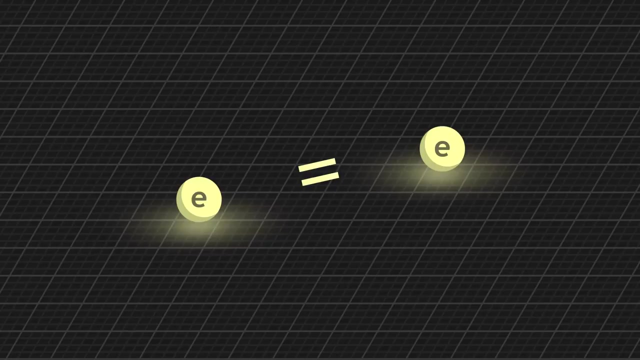 in nature. we often observe that particles can appear or disappear, like when a photon gets absorbed by an electron in an atom. Secondly, quantum mechanics treats each particle independently. However, within a family of particles, such as electrons, all exhibit the same properties and behaviours. How is it that an electron coming from the far reaches? of the cosmos has exactly the same mass as a star? The answer is no, it only support it. How is it that an electron coming from the far reaches of the cosmos has exactly the same mass as a star? The answer is no, it only support it. However, in nature, we often 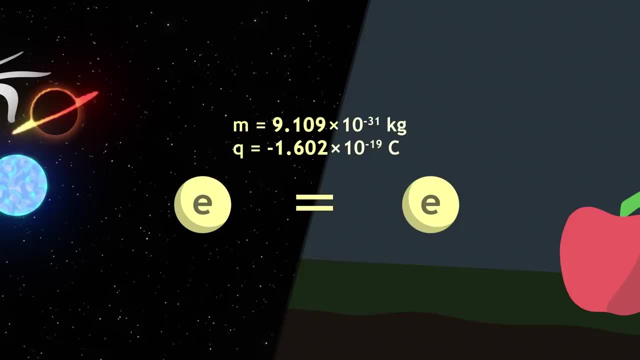 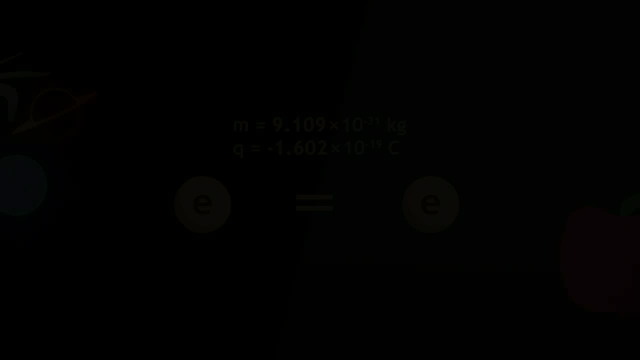 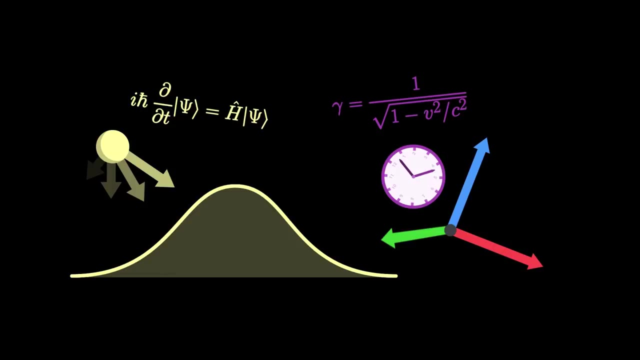 or charge as an electron in an apple? To answer this question, we will have to build a new mathematical framework, a more general description that reconciles quantum mechanics with special relativity. We will construct the most successful framework available for describing the microscopic world. 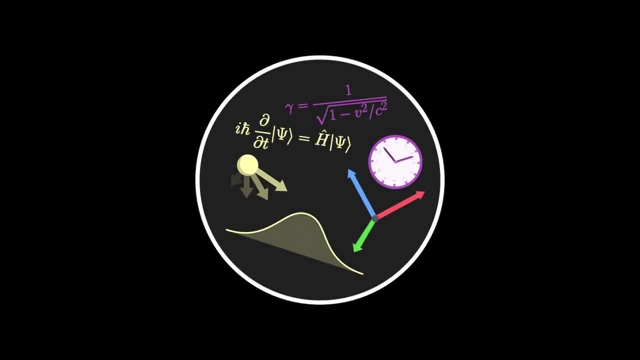 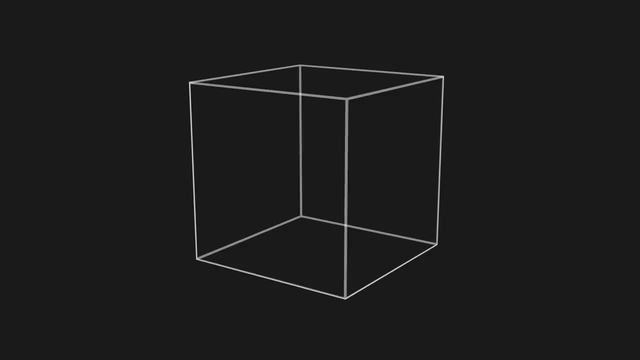 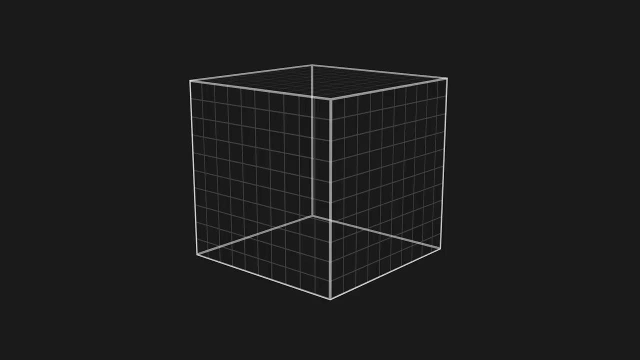 In this video, we build together quantum field theory. To begin with, let's start with an empty universe. Relativity teaches us that the fabric of the universe is space-time. To simplify, we will represent only two dimensions of space, as well as the dimension of time. 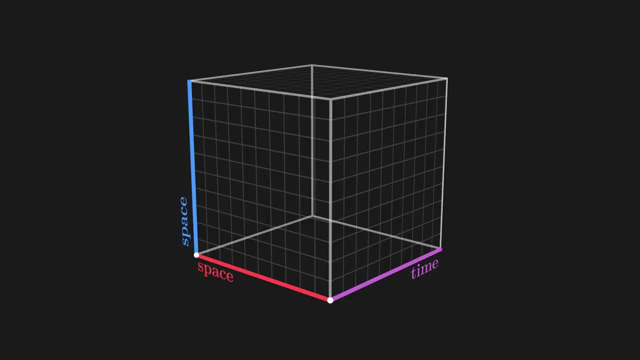 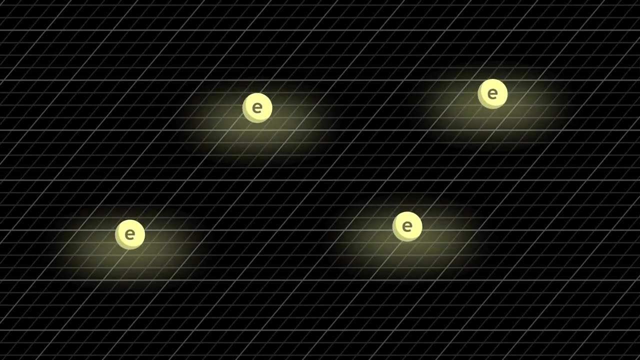 We now want to fill our universe with content matter. We saw previously that all particles of the same type, for example all electrons, appear perfectly identical, As if they were only the same. They are only local manifestations of a single underlying object which would fill the whole. 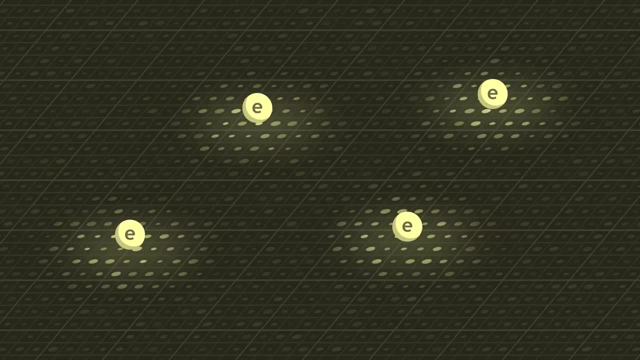 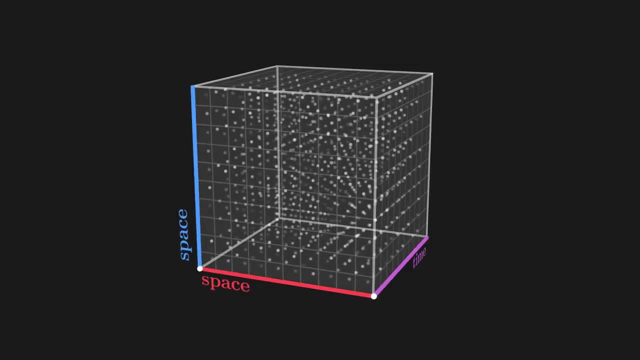 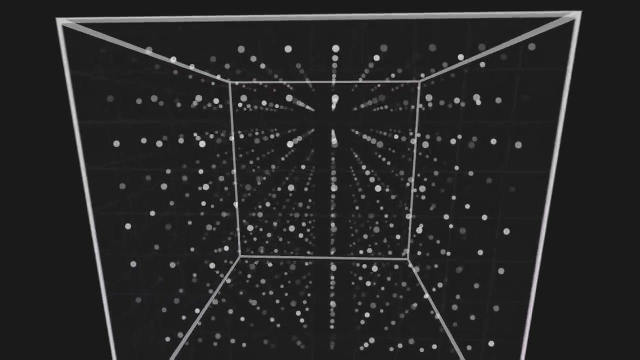 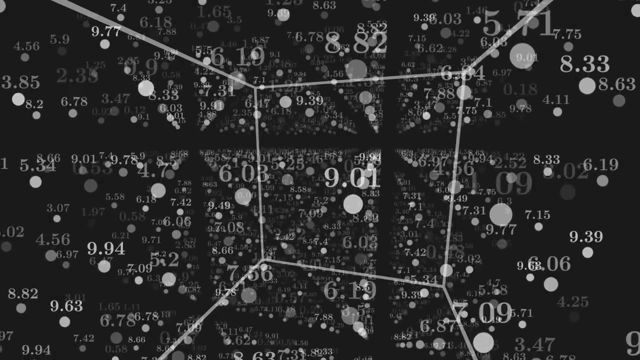 universe, A field To add content to our universe. we will therefore start by adding a field. In mathematics, a field is like a fluid which fills all space-time, each point of which is populated by a mathematical object. It can be a field of numbers. 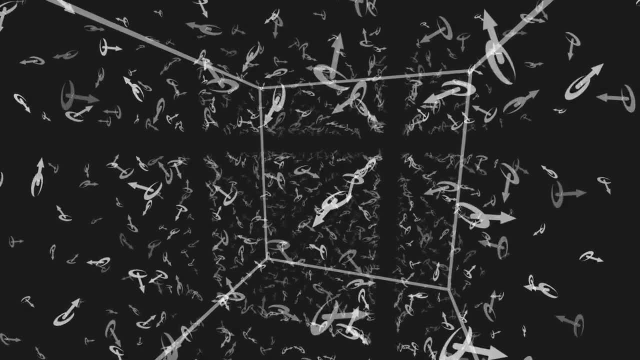 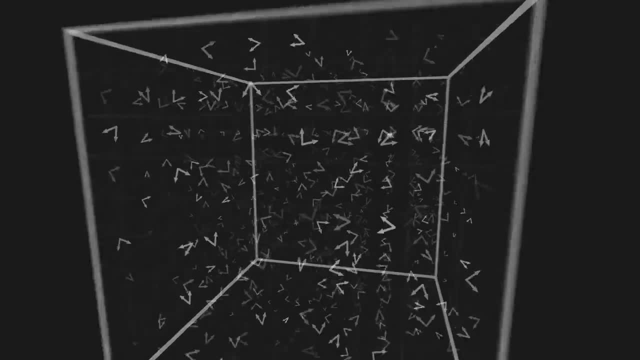 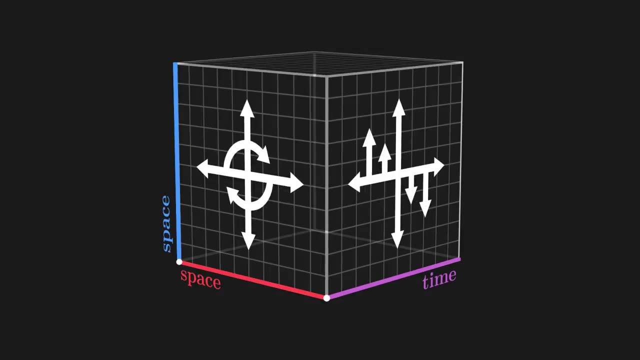 Vectors Or other more exotic objects. That said, special relativity imposes some restrictions. It forces us to respect certain symmetries which correspond to the geometry of space-time, Symmetries of translation, rotation or changing frame of reference. 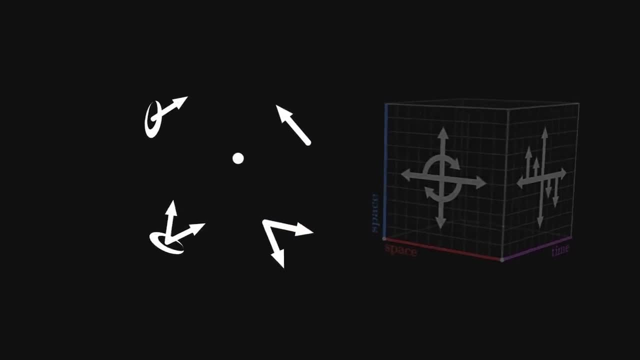 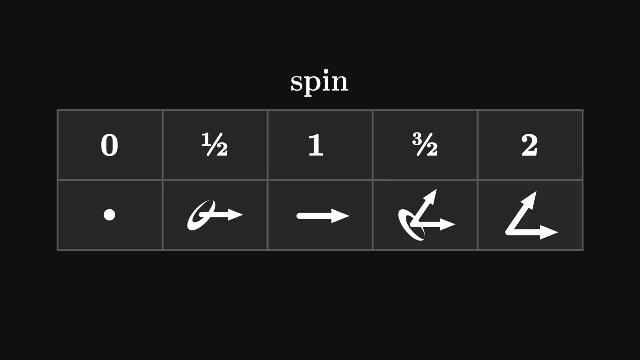 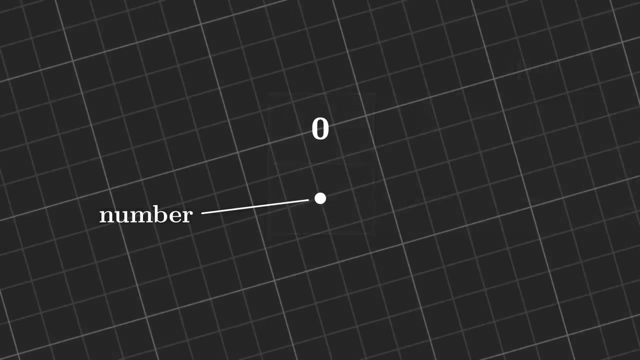 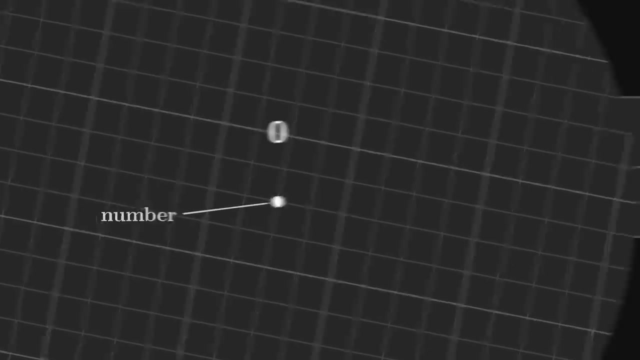 These symmetries are only respected by symmetry. They are not related to the geometry of space-time, But we are thats. Vectors, on the other hand, indicate a direction in space. The appearance of these objects depends on the orientation in which they are observed. They change their direction as they move or rotate, and they are thus bound to each other. They are not twenty-two-thousandth-inch-thousandth-inch-thousand-thousand-thousand-thousand-thousands-thousands- gursey-sum- helmet-like objects. 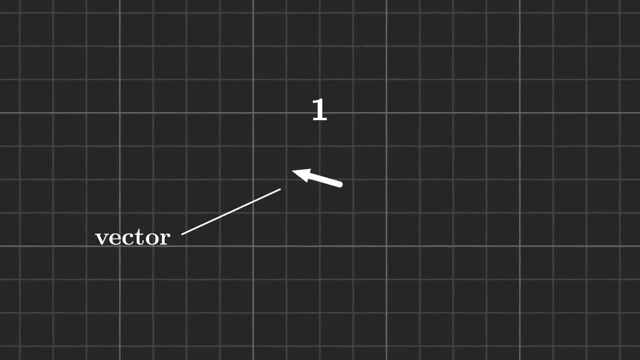 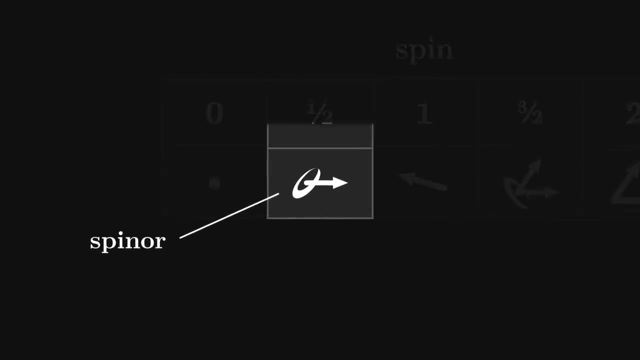 they are observed. We assign them spin 1 because when we rotate space by a full turn, a vector also describes a full turn. Finally, relativity also allows other, more exotic objects and in particular spinners, which have spin ½. You have to make two turns around a spinner. 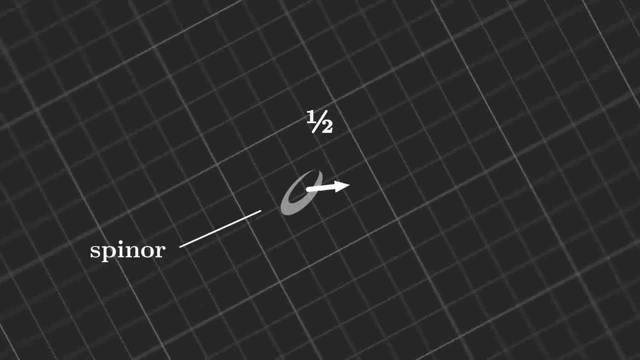 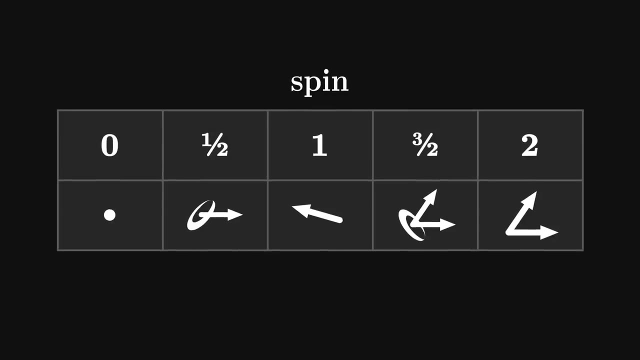 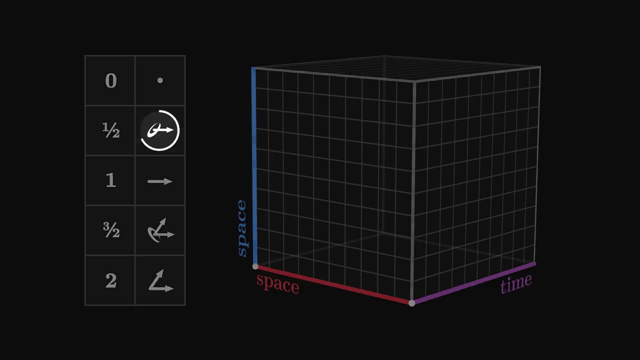 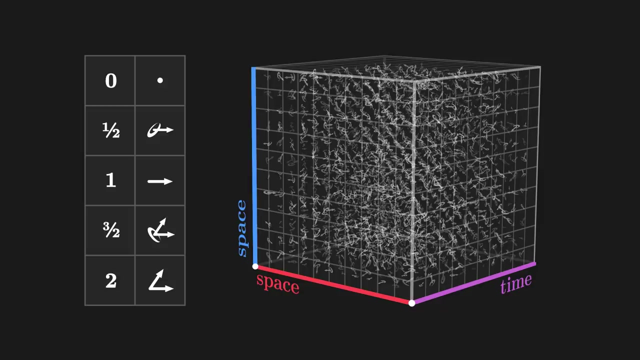 for it to come back to its initial state. All these mathematical objects seem very abstract and some are difficult to understand, but technically they all obey the symmetries of relativity and are therefore potential candidates with which we could fill our universe. 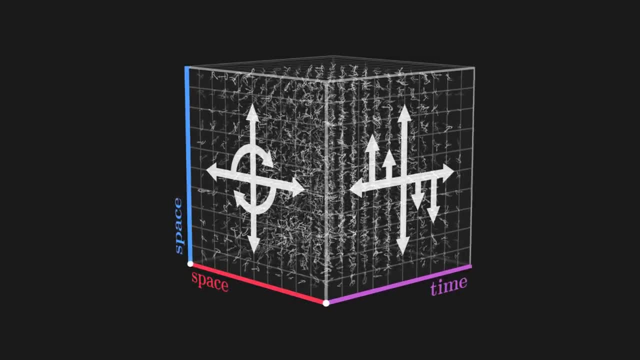 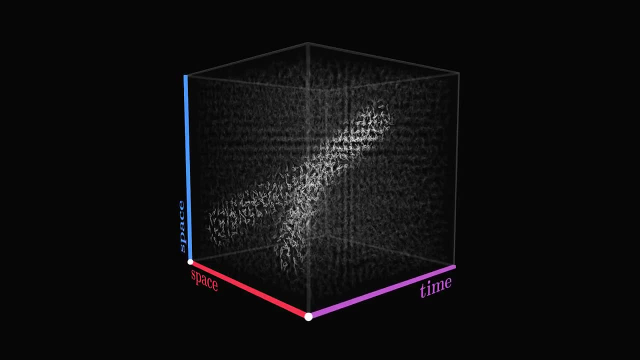 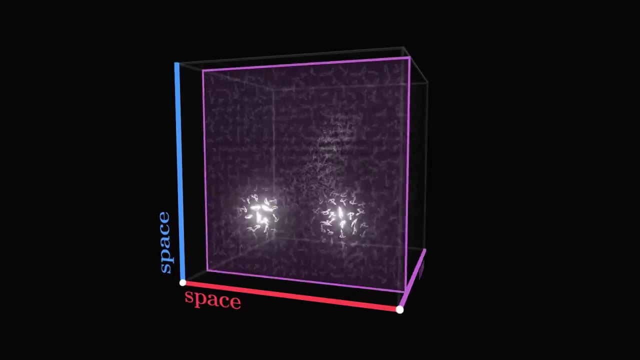 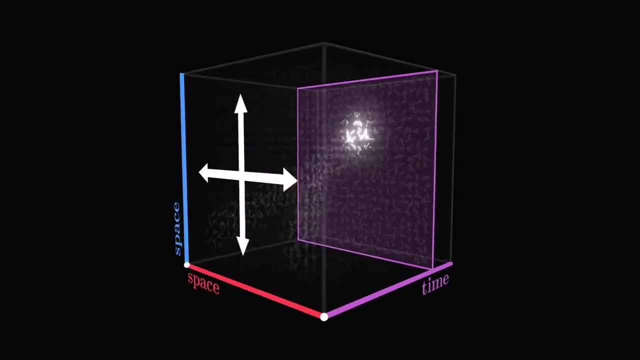 In addition to imposing the types of objects that are allowed spacetime, symmetries also set restrictions on the way objects behave inside the field. Each symmetry forces the field to respect the conservation of certain quantity over time, To obey relativity. our field must respect the conservation of energy momentum, angular momentum and velocity of. 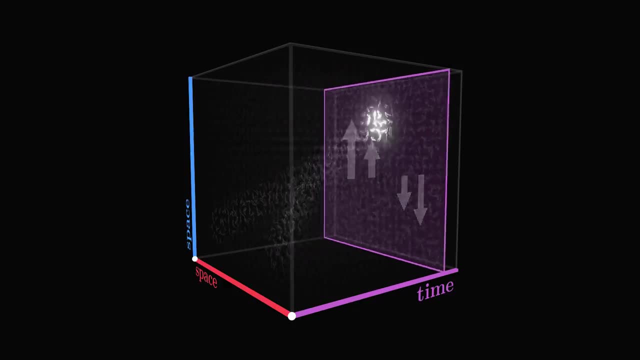 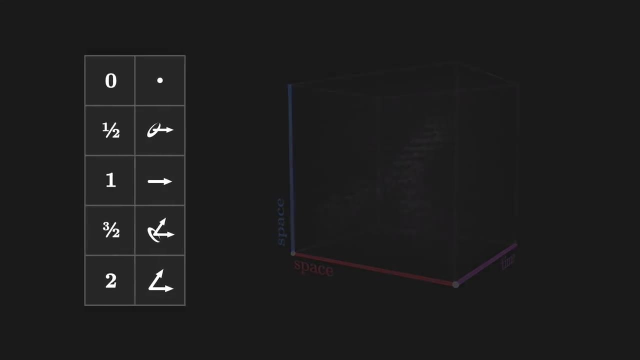 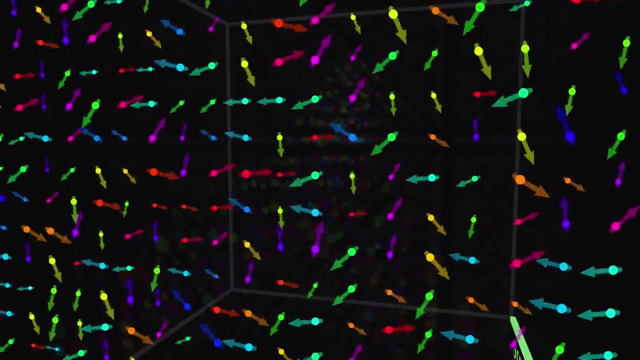 the centre of mass. Moreover, the mathematical objects themselves can contain symmetries of their own. If we decide to form a field with complex numbers, for example, they exhibit an internal symmetry which implies the conservation of another quantity over time related to the 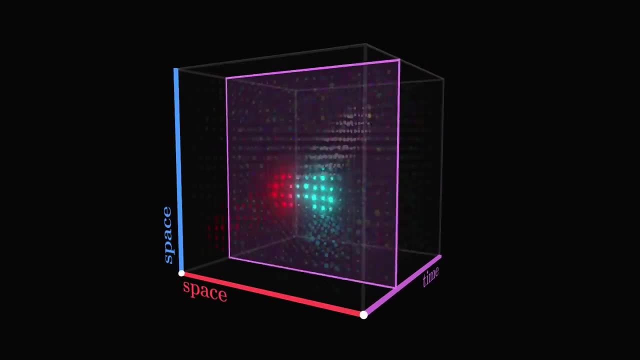 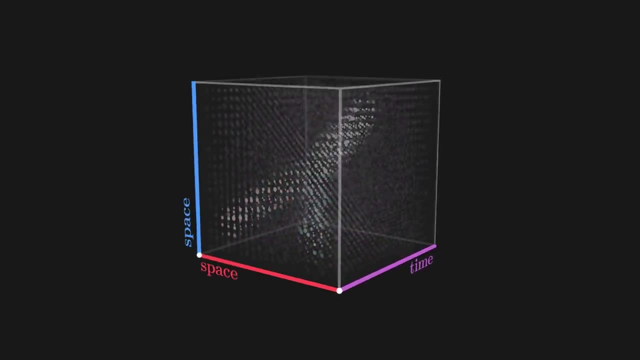 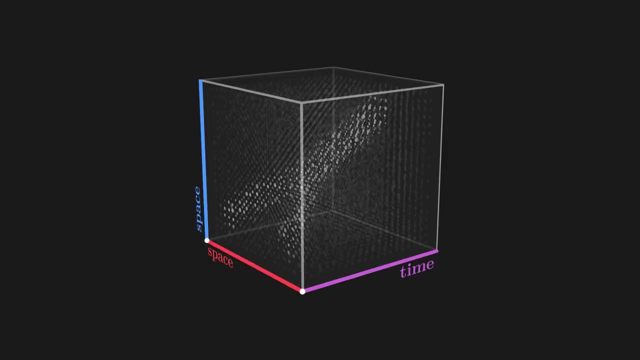 very nature of complex numbers, the electric charge. At this stage we have a spacetime which we have filled with a field which satisfies all the restrictions imposed by special relativity. But are we really going to be able to do that? If we do, then we are going to be able to do. 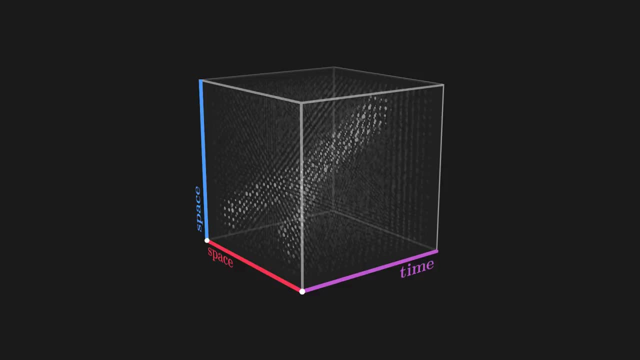 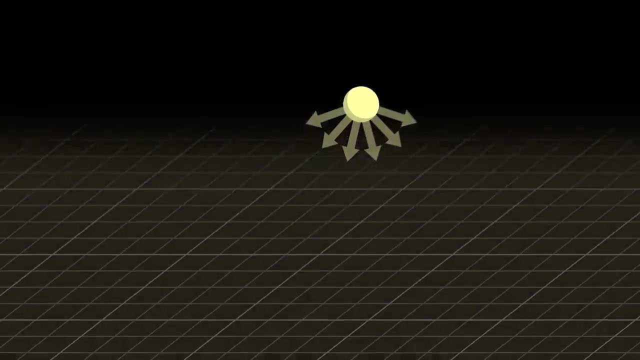 it. Our goal is to describe the microscopic world, so it's time to turn our field into a quantum field. In quantum mechanics, to transform a classical object into a quantum object, we allowed it to adopt several positions at the same time, with more or less probability. 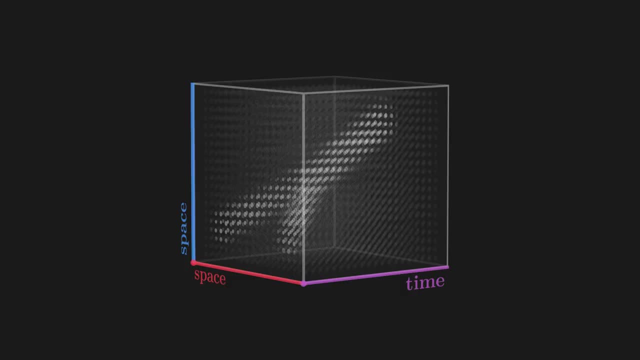 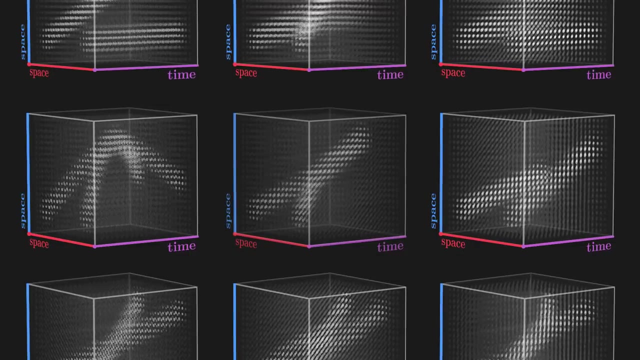 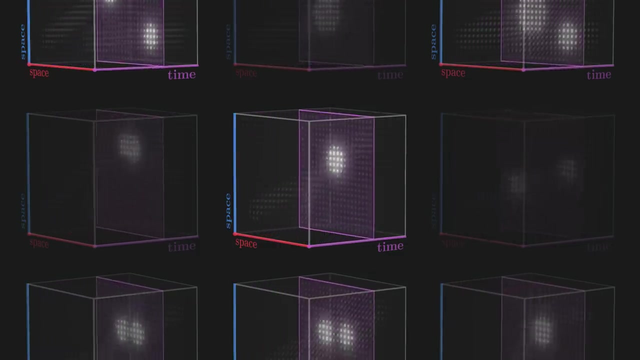 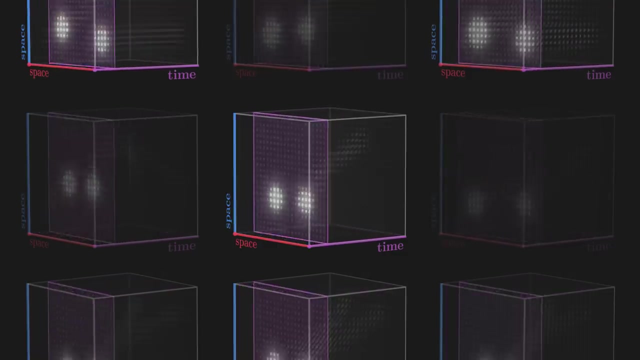 Similarly to transform a classical field into a quantum field. we allow it to adopt several configurations, Multiple ways. it can evolve with more or less importance Over time. our field evolves as a superposition of all possible scenarios. Transitioning from a classical field to a quantum field results in a very interesting 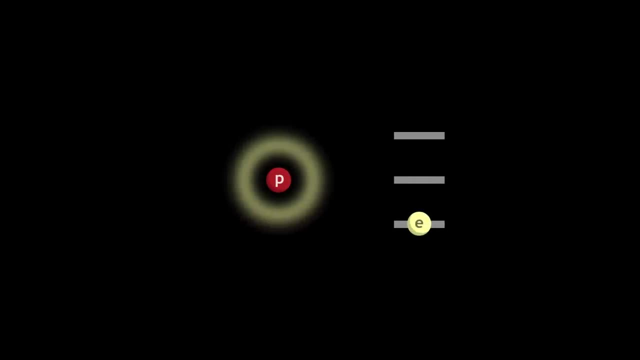 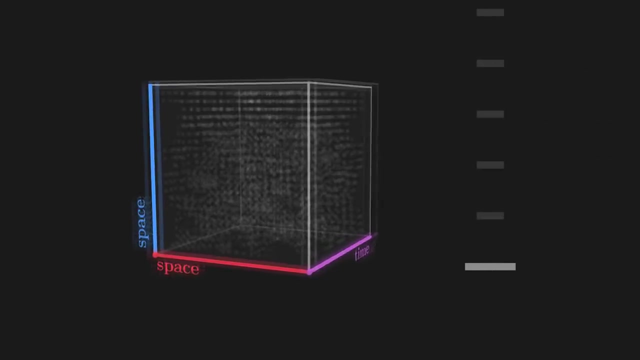 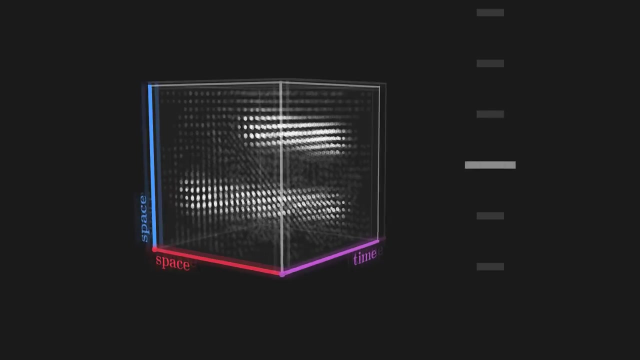 property. Just like an electron in an atom has well-defined energy levels, a quantum field has well-defined energy levels. A quantum field also has energy levels. It can only contain an integer number of disturbances, quanta of energy that can appear or disappear. 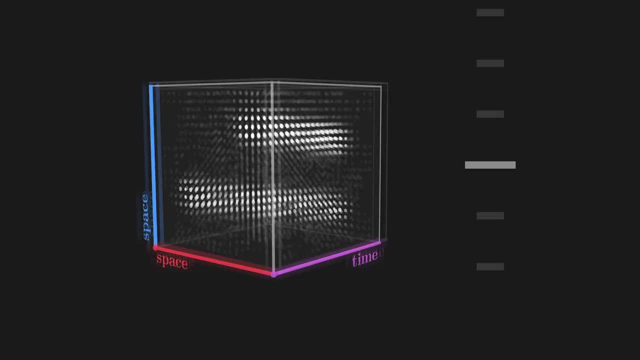 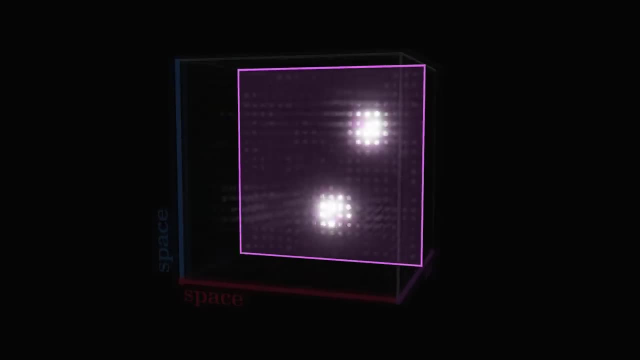 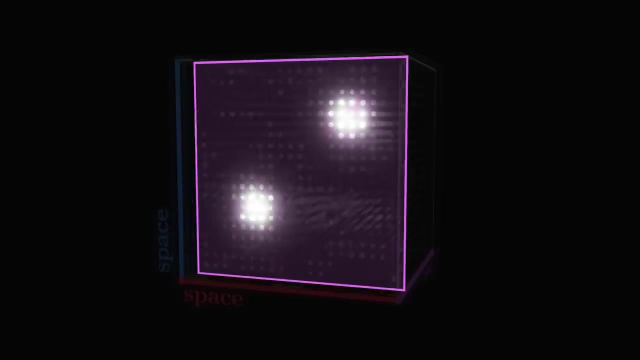 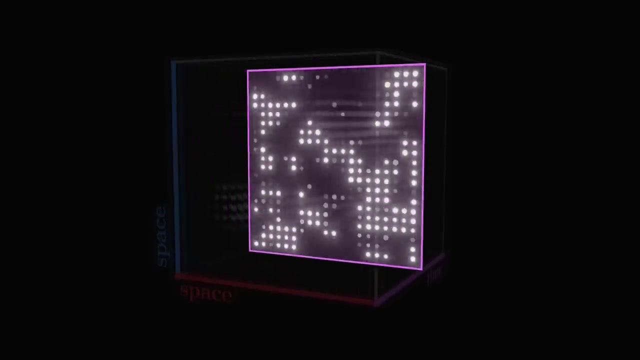 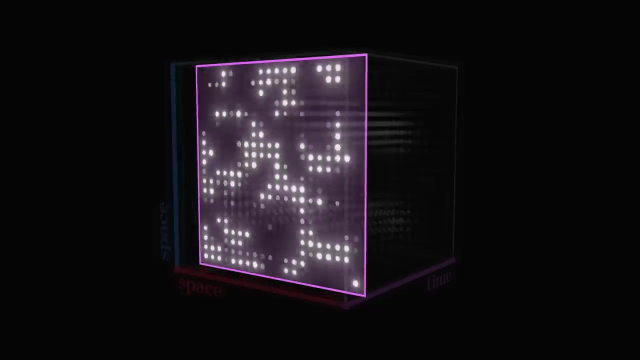 These are particles. Much like a wave on the surface of water, a particle is simply a disturbance which propagates within the field. A quantum field is also agitated by fluctuations. These are called virtual particles. These virtual particles exist only very briefly, so that it is strictly impossible to observe. 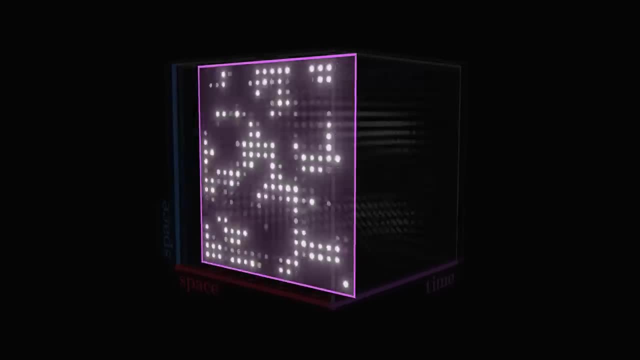 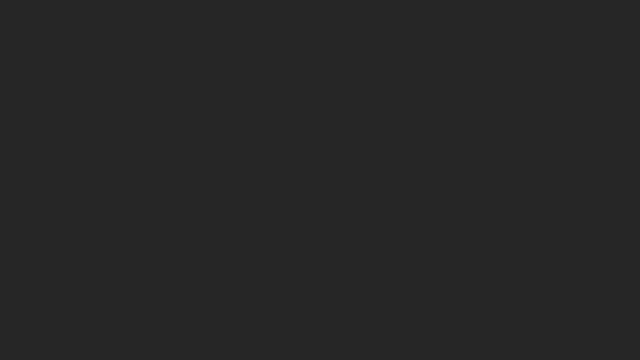 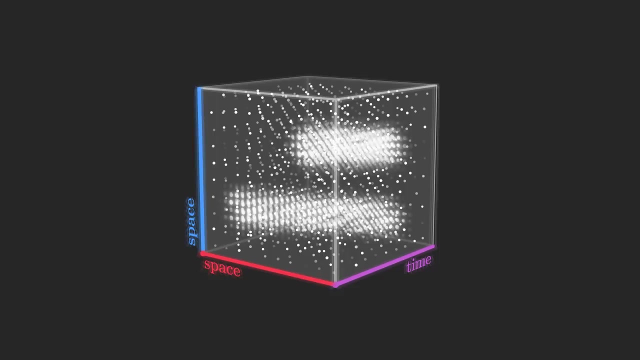 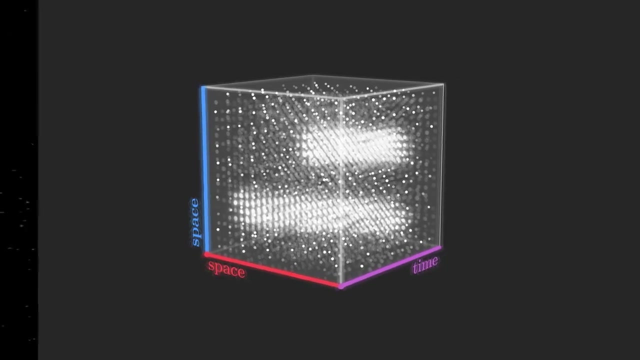 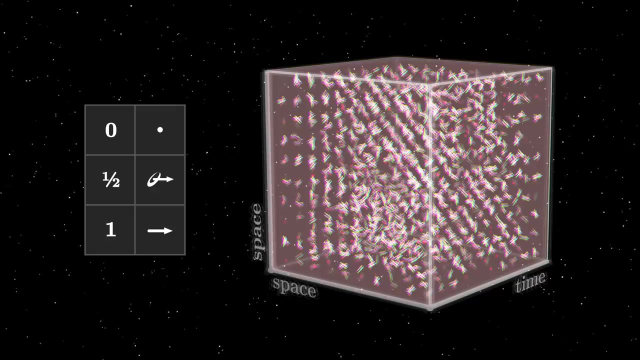 them Step by step. our model universe is getting closer to reality. inside which move disturbances, particles in a soup of fluctuations, virtual particles. In our universe, several fields coexist and constitute different families of particles. Some are vector fields, spin-1,, and the particles they contain are photons, z and w bosons. 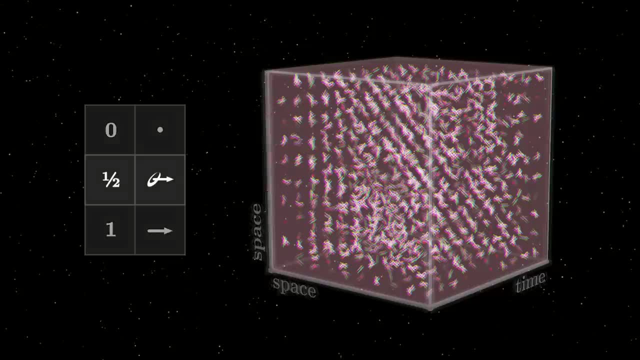 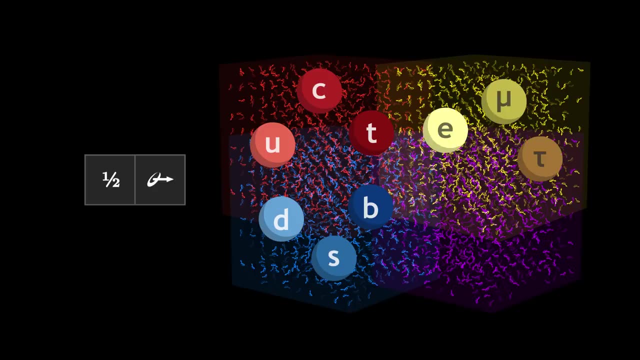 and gluons. Others are fields of spinners, spin-1⁄2.. They are the fermions that make up matter: Quarks, electrons, muons, tau particles and neutrinos. Finally, there is a field of spin-0,, the Higgs field. 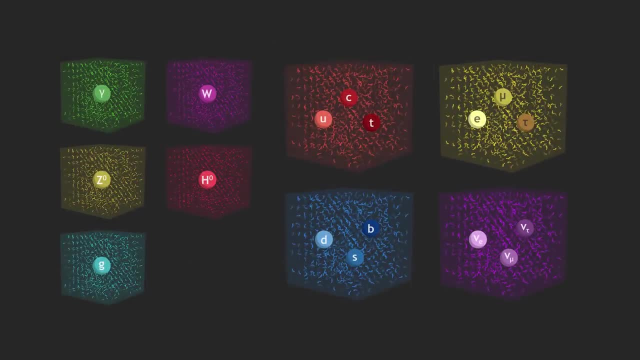 Among all these fields, most have internal symmetries which provide them with quantities that are conserved over time. Charges which distinguish their particles between c and d help them see which of these is true. Also, as a matter of fact, many of the objects 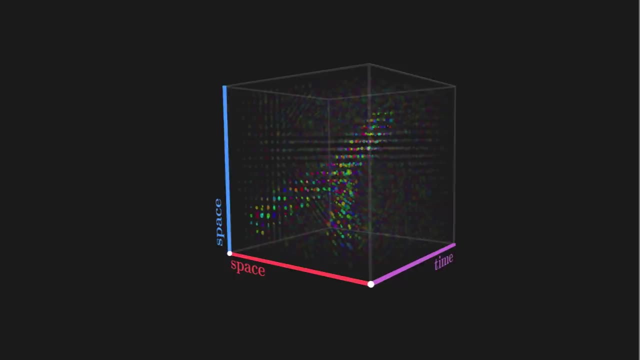 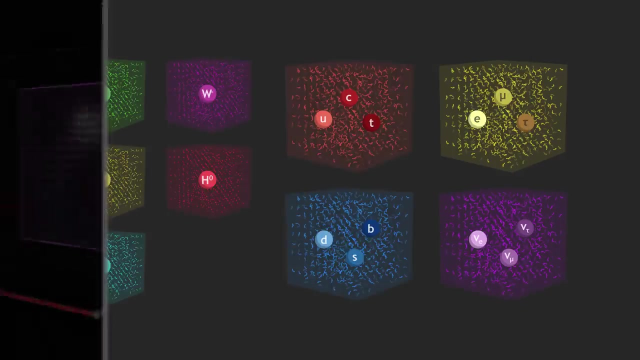 in this world are the same. They differ in structure, how they work and how they move. several versions. We saw previously that fields formed with complex numbers have a symmetry which gives them their electric charge. This symmetry allows us to distinguish two versions. 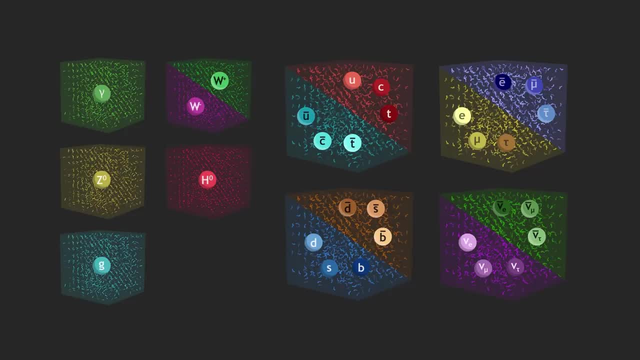 of the particles, one with positive charge, the other with negative charge. This is antimatter. In a way. the antiparticle is the complex conjugate of the ordinary particle. Other fields also have more exotic symmetries. The quark fields, for example, exhibit a symmetry. 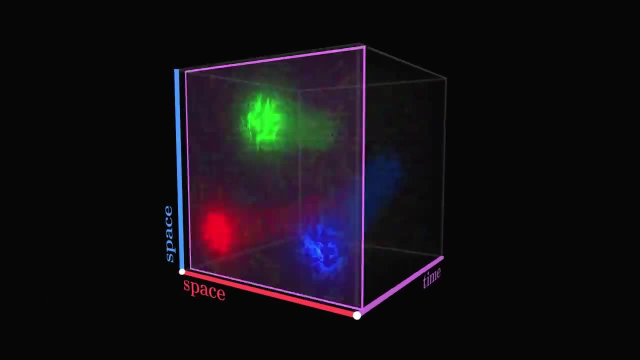 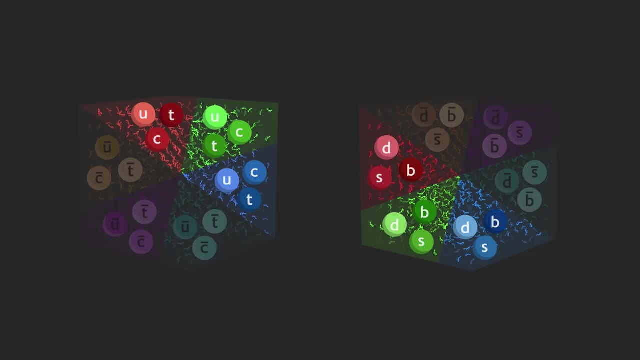 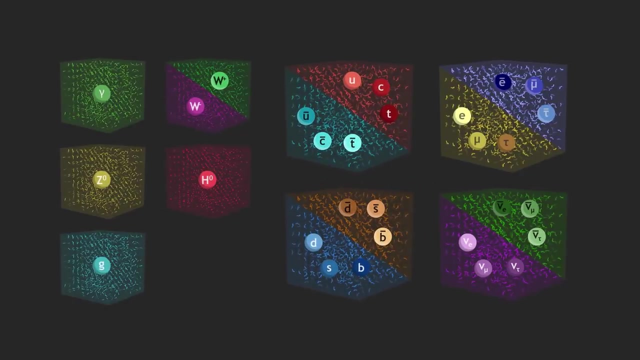 which assigns them another charge, the colour charge, which must also be conserved over time, and that allows us to separate quarks into three versions: red, green and blue. The set of all these fields that make up the content of our universe is the standard model. 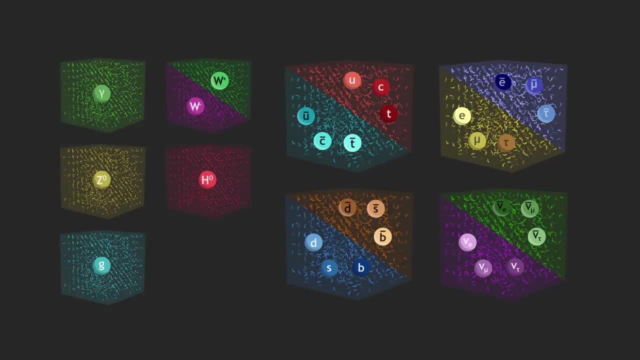 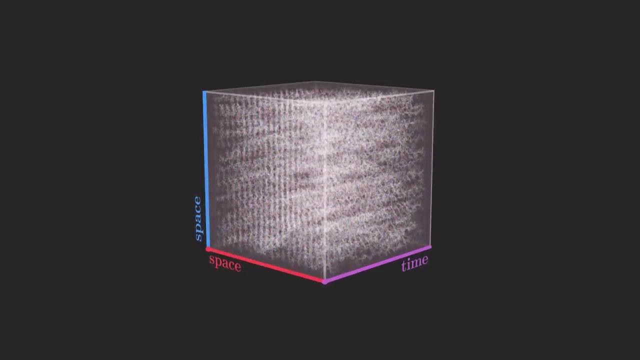 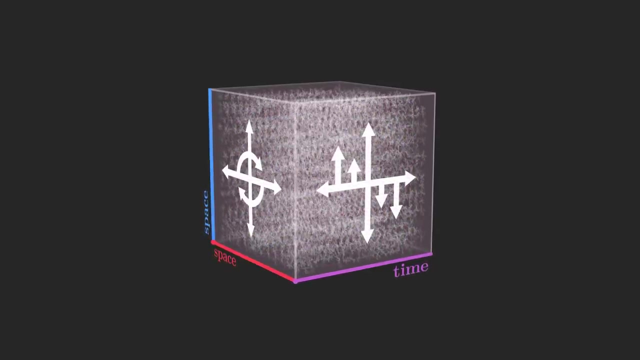 of particle physics To this day. this is the most successful description of our universe on the microscopic scale. Our model universe now contains the same particles as our real universe. However, it still isn't realistic. Indeed, the symmetries of space-time force all particles to move in straight lines. 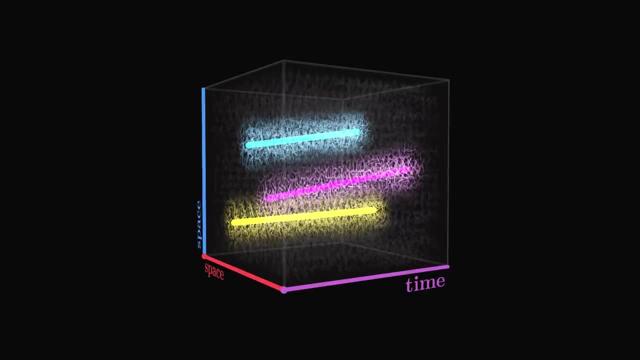 forever, independently one from the other. To finally complete our model, all we have to do is add one more fundamental ingredient. We need to allow these fields to interact with each other. To understand, let's focus on one of the simplest interactions between the photon. 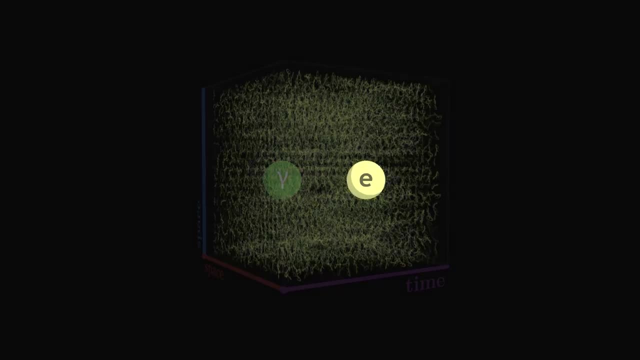 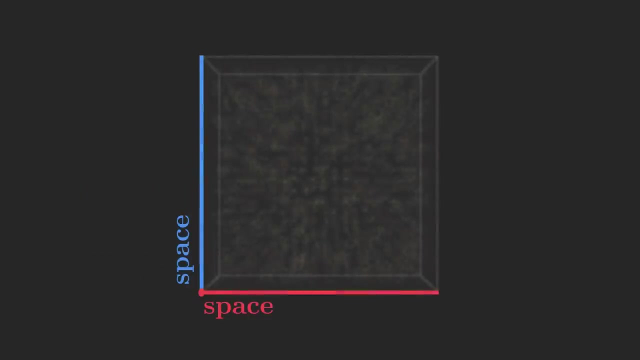 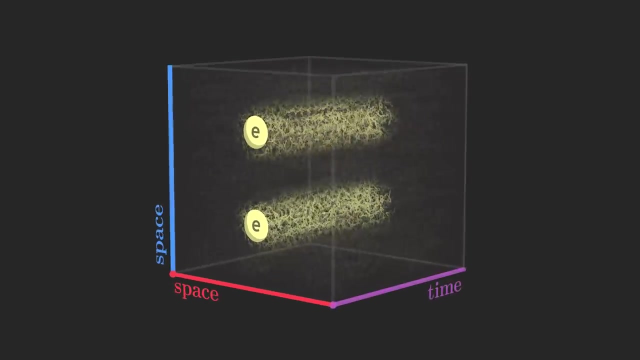 field and the electron field. We will allow an electron to emit or absorb a virtual photon and vice versa. Allowing only this simple interaction will have drastic consequences. for instance, in the following situation: We start with two electrons motionless. Over time, the two electrons progress towards. 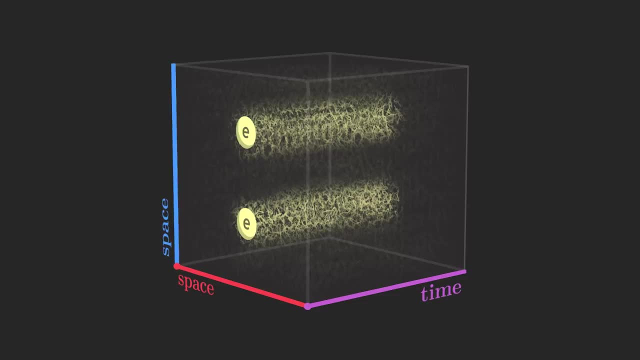 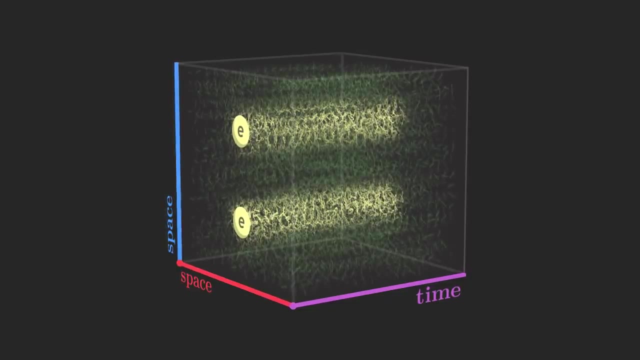 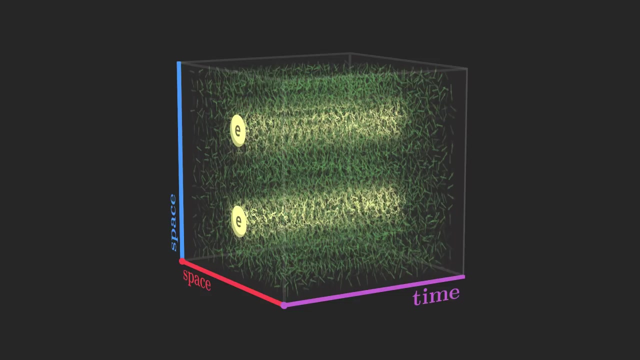 the future. At first one might think that the two electrons remain motionless indefinitely, But that would be forgetting that our electrons are constantly moving through the photon field with which we allowed them to interact. We saw that a quantum field realises all possible. 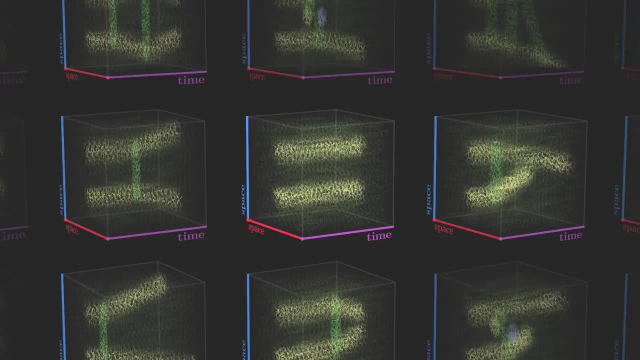 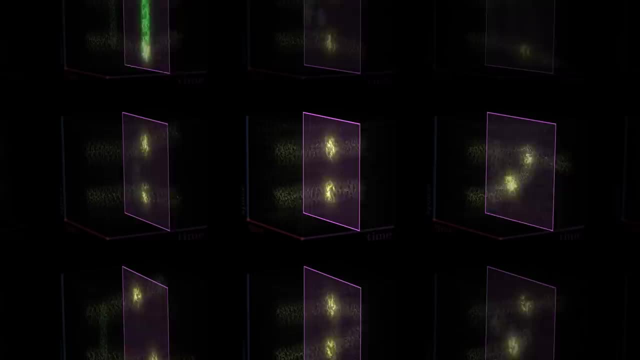 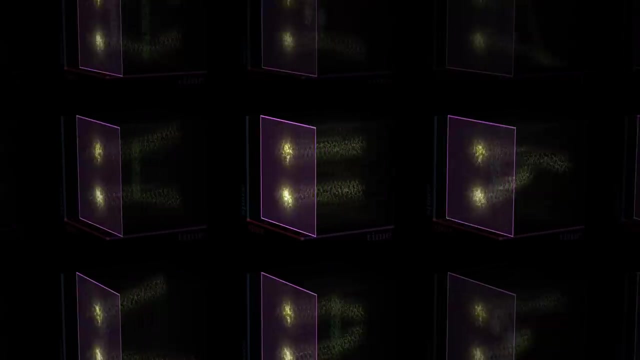 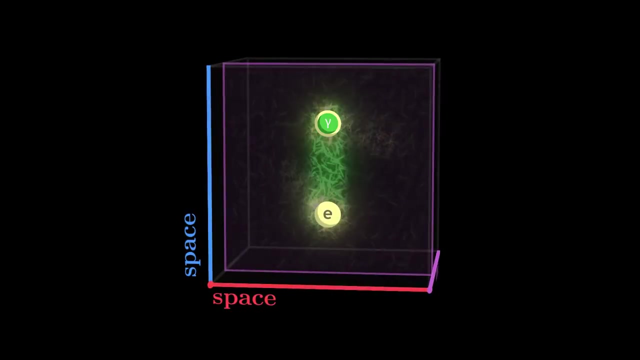 In a way, each evolution describes a scenario, and in some of these scenarios the electrons will interact with the photon field. In this scenario, for example, the electron emits a virtual photon at a certain instant which carries away part of its momentum, and the virtual photon is absorbed a little later. 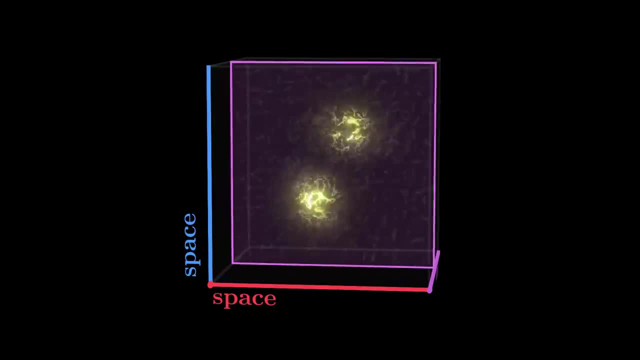 by the other electron, We see that the electron is absorbed by the other electron. in this other scenario, the electrons exchange, this time two photons. or again in this third, more complex scenario, the electron emits a virtual photon, which is converted into a pair of virtual electron and positron that annihilate 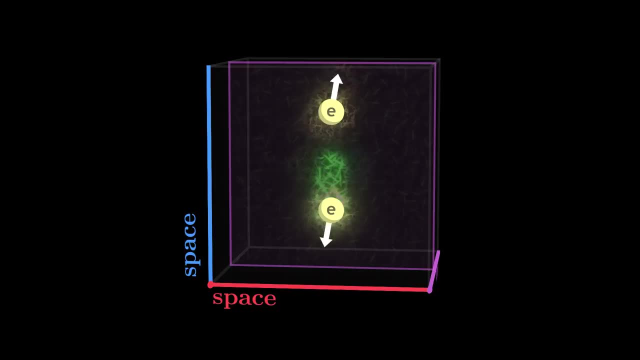 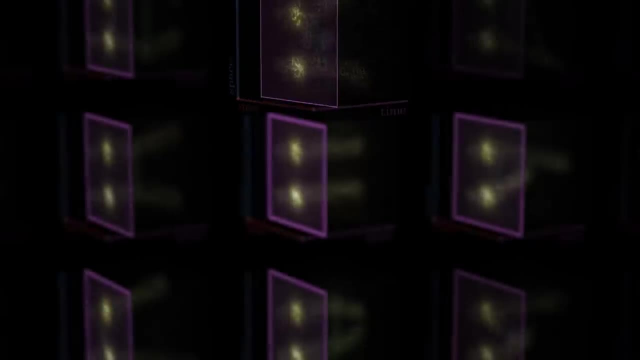 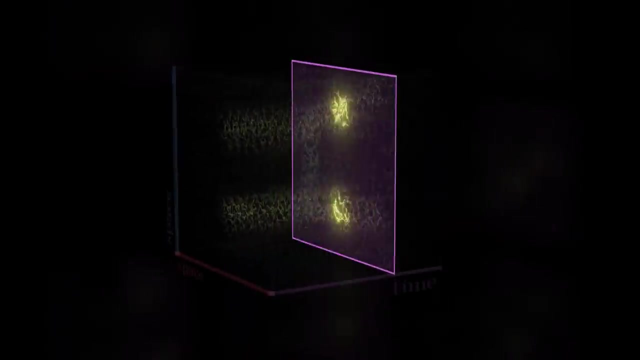 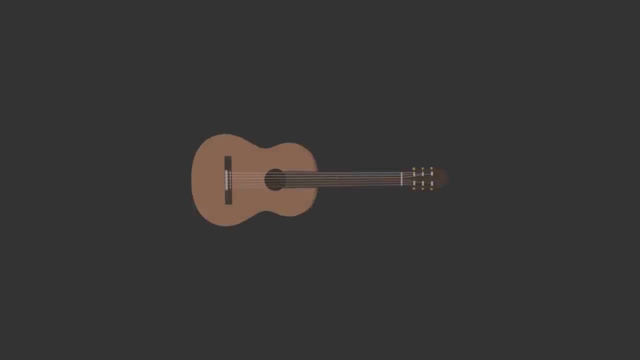 together into a virtual photon, which finally ends up absorbed by the second electron. by exchanging part of their momentum, carried by virtual particles, the two electrons will, in some scenarios, get closer and in others, get further apart. now consider the following analogy: on a guitar, a string can vibrate with. 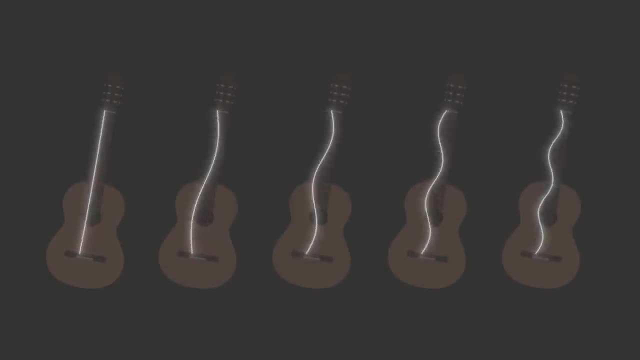 different frequencies, each of which corresponds to a pure sound, but when we pluck the string, it starts to vibrate in a different way. it can vibrate in a superposition of all these frequencies, with more or less amplitude, and the synthesis of all these pure sounds, together with different 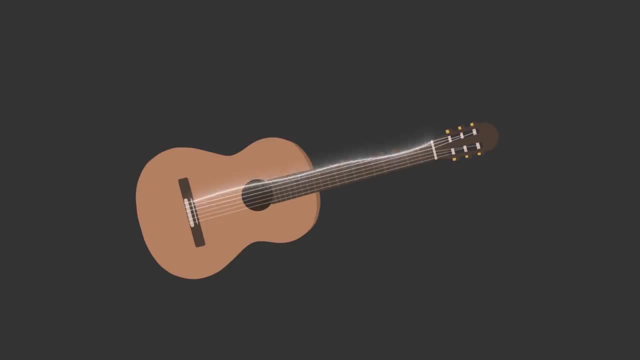 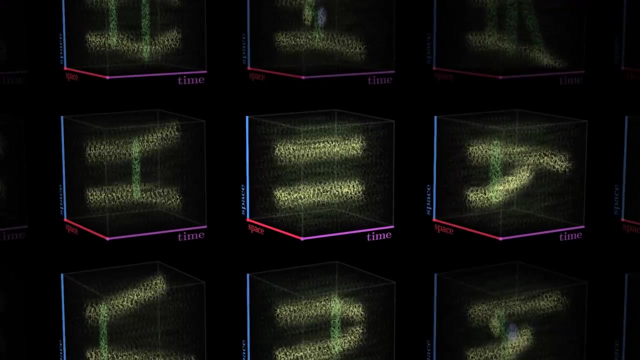 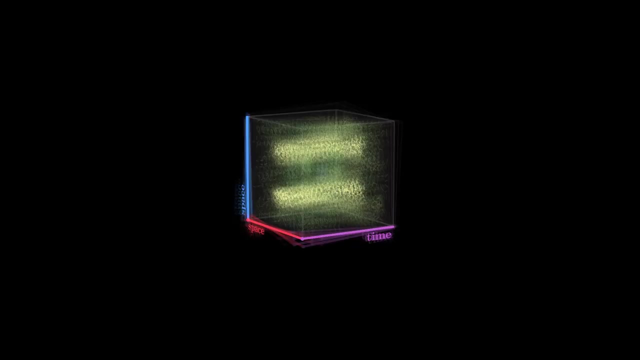 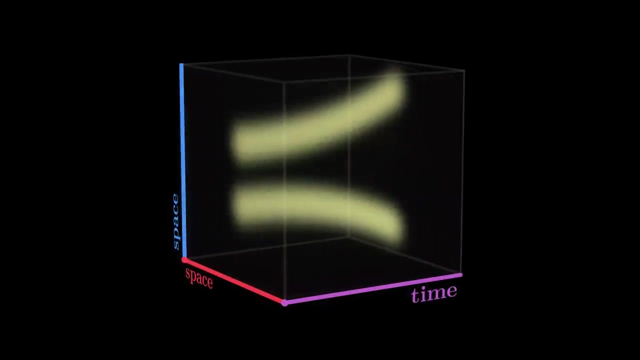 amplitudes is what makes the total sound produced by the string. similarly, a quantum field evolves according to every possible scenario, with more or less amplitude, and it is the synthesis of all these scenarios together that describe the real evolution of the physical system, in particular in our example. when we add up all these possibilities, we observe that, overall, 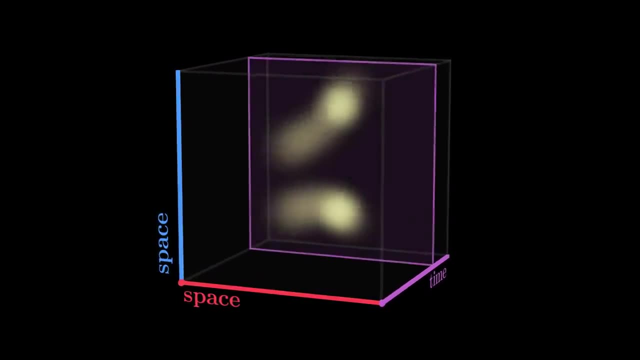 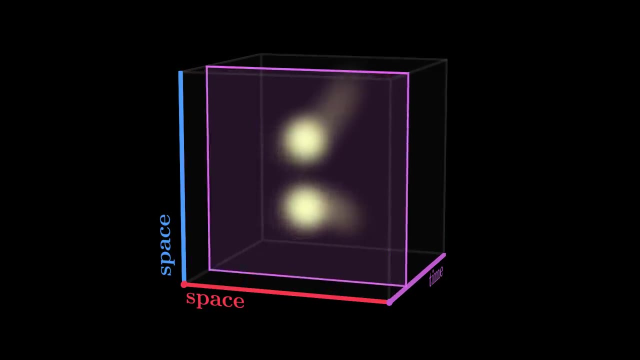 our two electrons are more and more deflected. they feel a force repelling them because of the exchanges of virtual photons. this is the electromagnetic force, and if, instead, we had started with an electron and a positron of opposite charge, the amplitudes of the different scenarios would have been different. 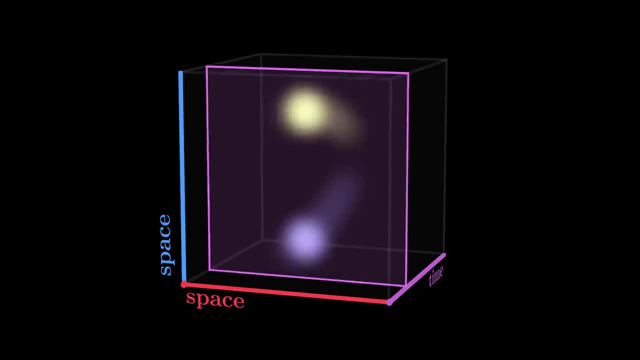 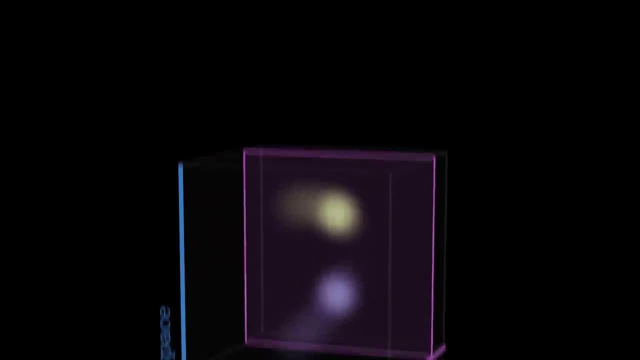 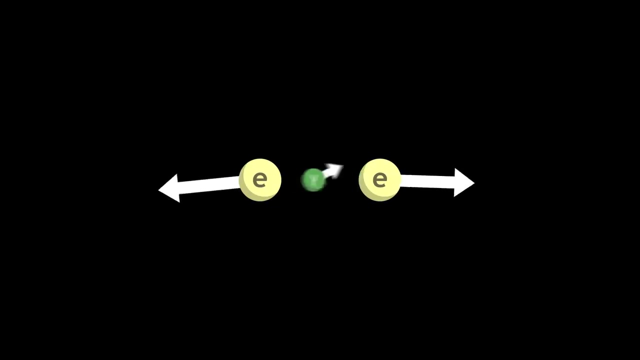 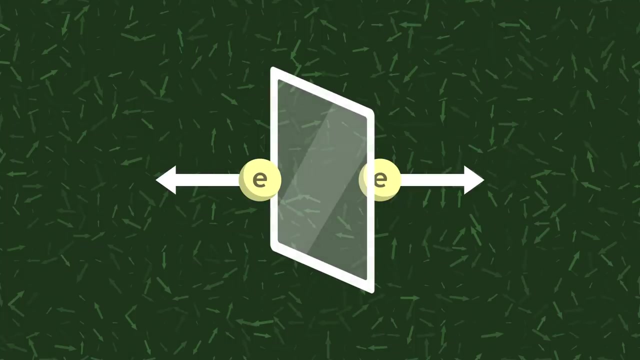 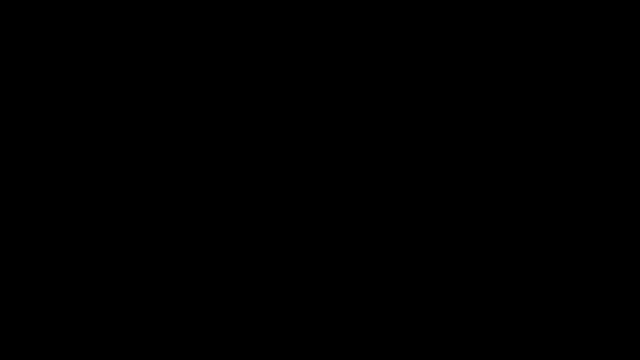 resulting this time in an overall attraction force. by allowing particles to interact and exchange momentum, quantum field theory explains how forces arise from simple symmetry's: the symmetries of the fields which make up our universe. to conclude, quantum field theory is a mathematical recipe for building a model universe. 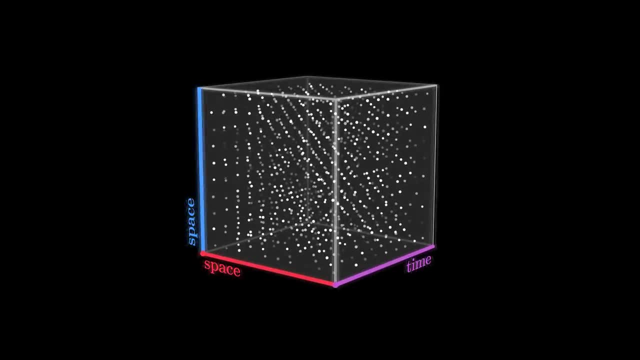 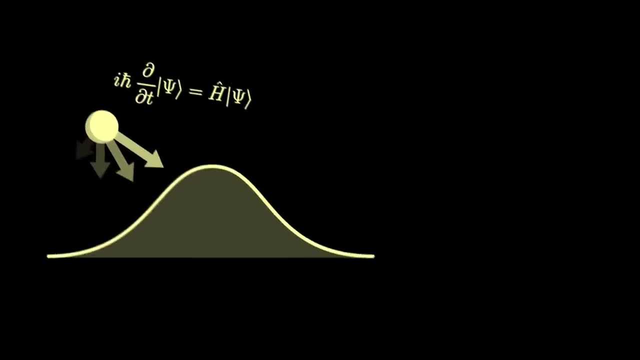 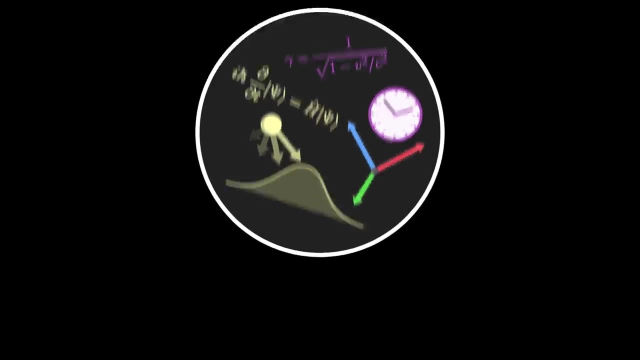 We start with an empty space-time, which we fill with quantum fields that satisfy the symmetries of special relativity. Quantum field theory thus makes it possible to construct a quantum description of our universe which satisfies the constraints imposed by relativity. By allowing fields to interact with each other, this theory makes it possible to predict with 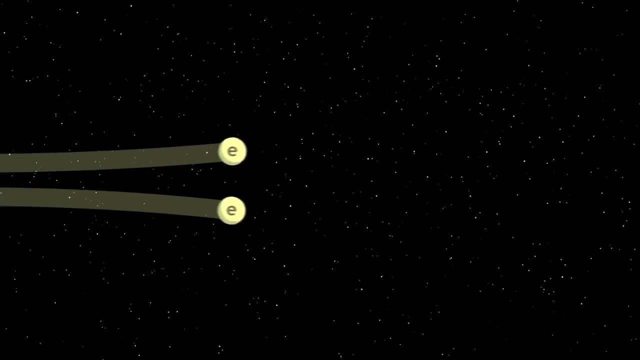 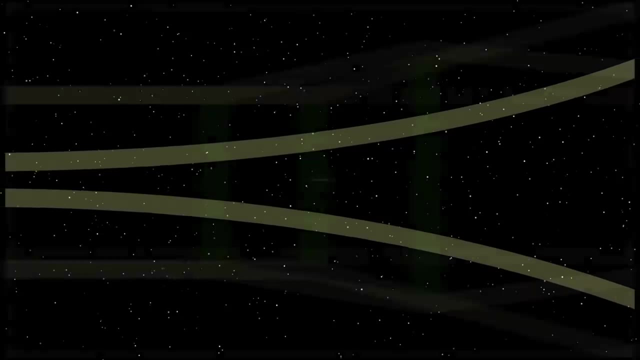 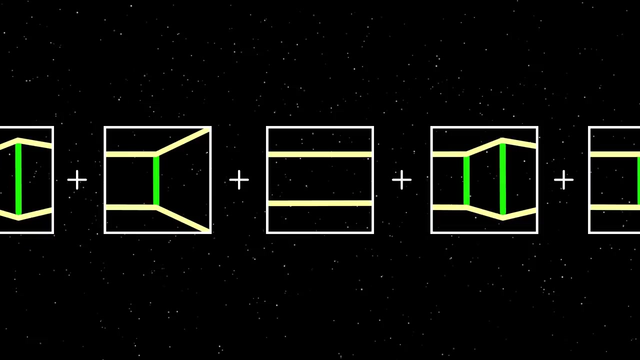 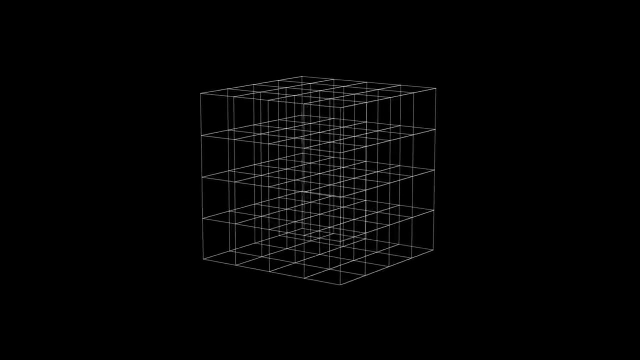 astounding precision the phenomena that govern our universe. According to quantum field theory, the evolution of our universe is described as the synthesis of all possible scenarios at the microscopic scale. That being said, this description remains incomplete as, even though it satisfies special relativity, quantum field theory cannot be unified with general relativity, which describes